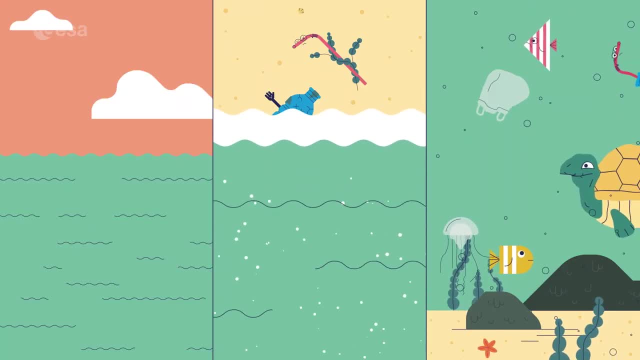 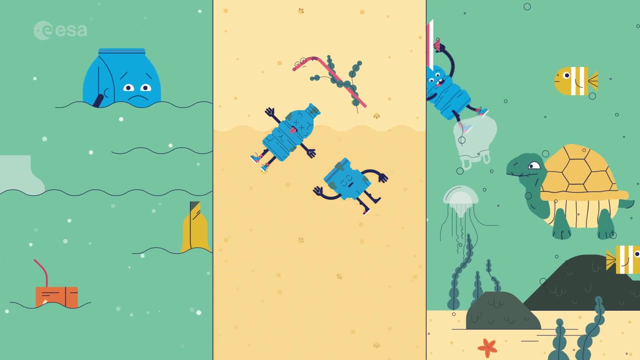 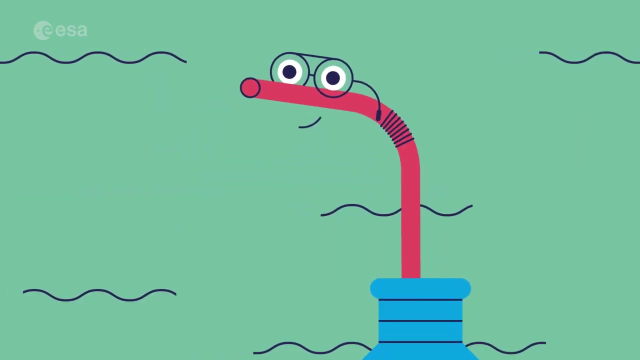 Here we go. Bag, Bottle and Straw could end up in the middle of the ocean or be washed up onto another beach where they would stay for hundreds of years, Or a sea animal could eat them, become sick or even die. Hey, look, What's that. 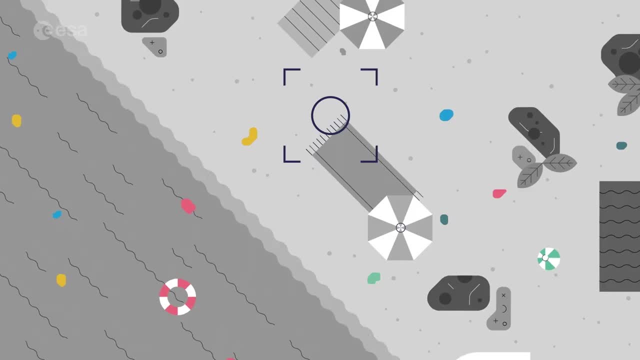 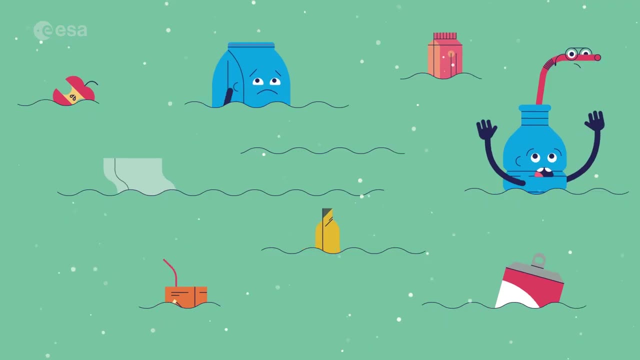 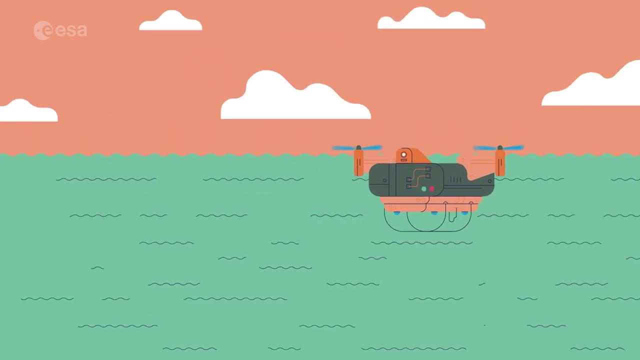 Drones use very good cameras to take photos of the plastic that is left on the beach or washed up there, But these three are already in the open ocean and they're really small. The drone can't see them. Not all plastic can be found with a camera anyway. 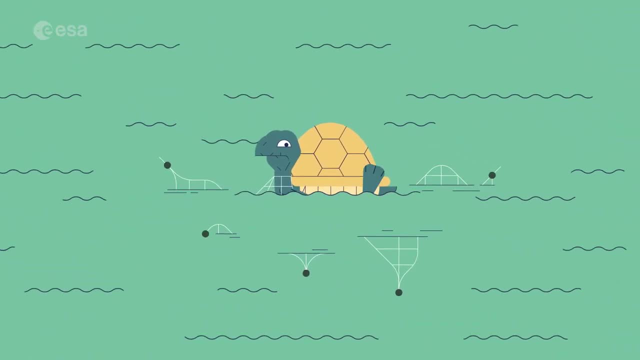 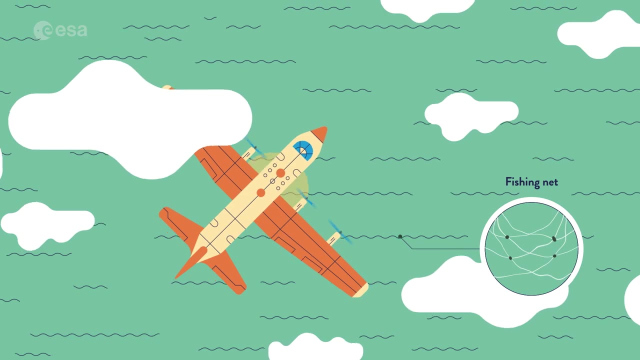 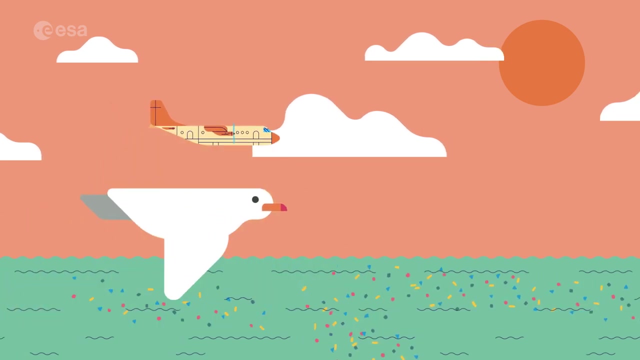 Take this lost fishing net. It's hard to see from above, and yet it can be a nightmare for sea animals. Planes use special cameras. Planes use special instruments to look for specific types of plastic like this net. They cover a larger area than drones. 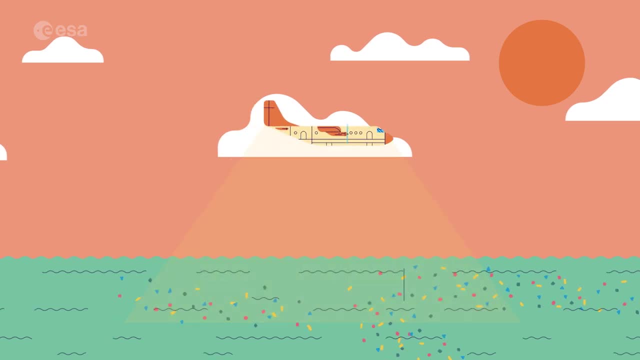 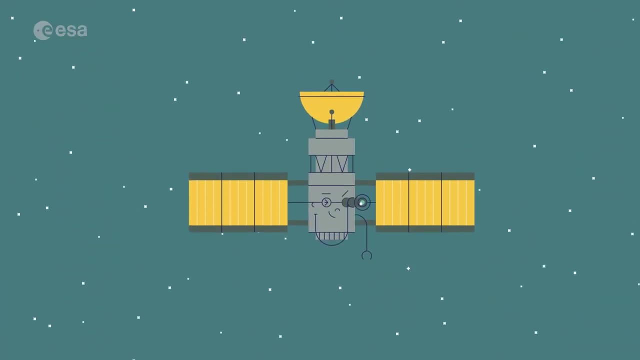 And they're great for spotting build-ups of plastic further from the coast. But there is something even higher up that can be used to spot and track ocean plastic. Meet one of our satellites. Hi, I'm Satellite. Right now, the European Space Agency is exploring how satellites can detect. 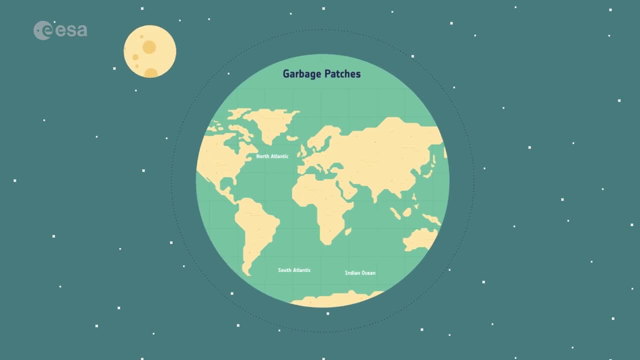 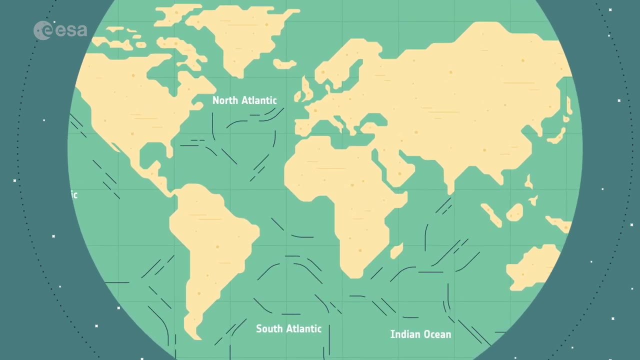 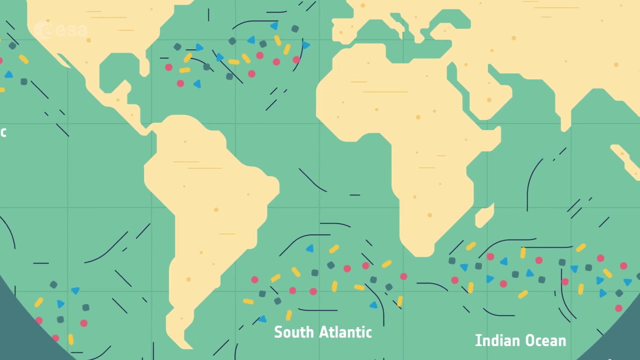 large build-ups of floating plastic. But that's not all. Pieces of plastic like bag, bottle and straw can be carried by ocean currents for thousands of kilometres. In some places, currents swirl around, trapping plastic and forming large build-ups. Gross right. 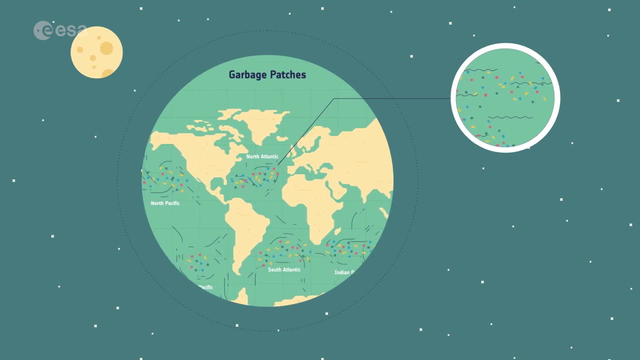 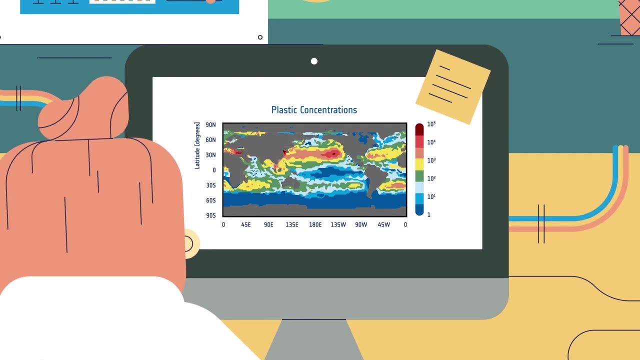 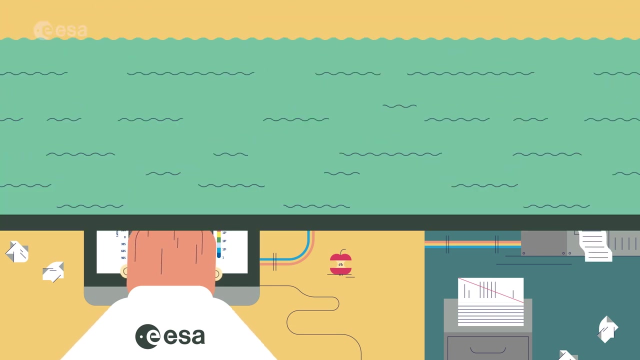 Satellites can spot big build-ups of plastic like this one, But they can also follow the currents that move plastic around the ocean. They send the information they collect down to scientists on Earth to help them understand where the plastic comes from, where it goes and where it ends up. 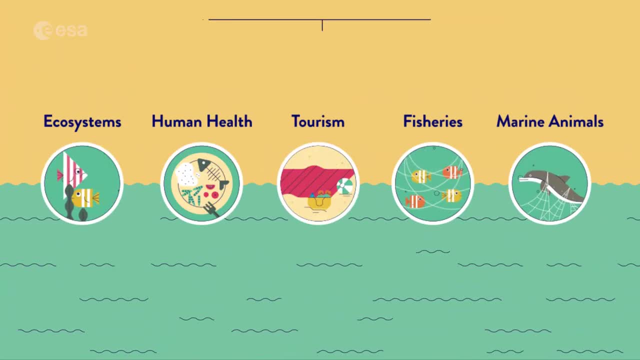 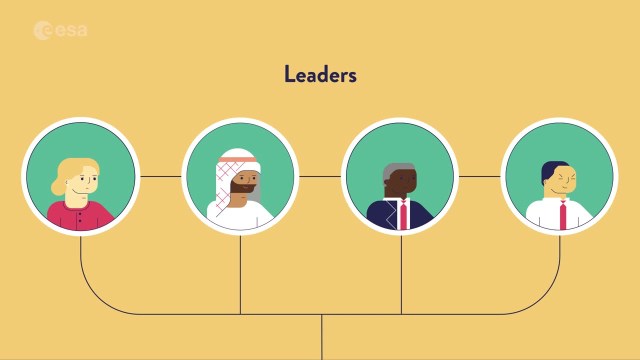 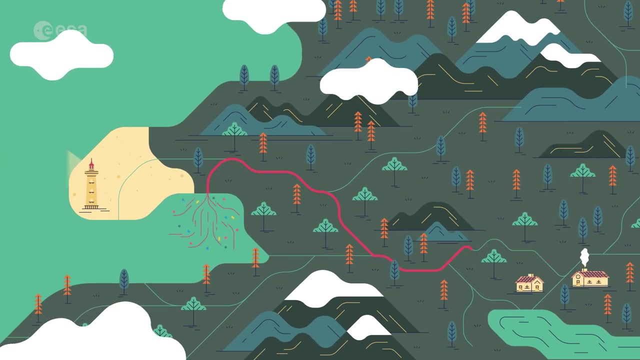 Using this information, scientists can help our leaders find solutions to the huge problem of plastic pollution and eventually reduce the harm that it causes. But the best way to avoid this harm is- you guessed it- if no plastic enters the ocean in the first place. 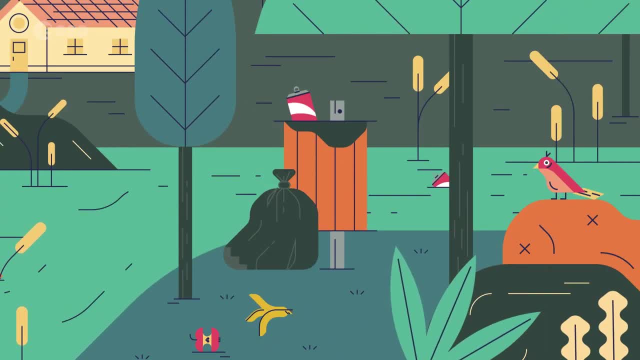 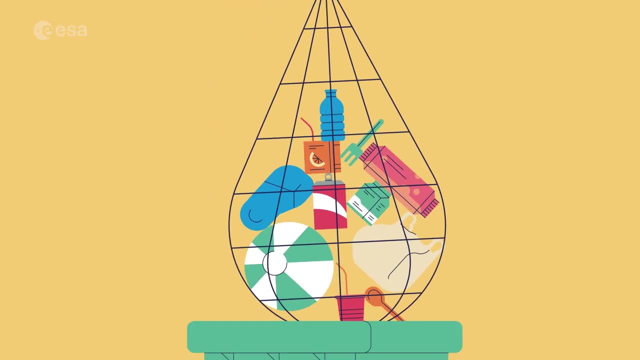 Even if you drop litter far from the ocean, it can be carried there by wind and rivers. So how about putting that plastic in the recycling bin? Or, even better, not using disposable plastic at all? How can we all follow the three R's?